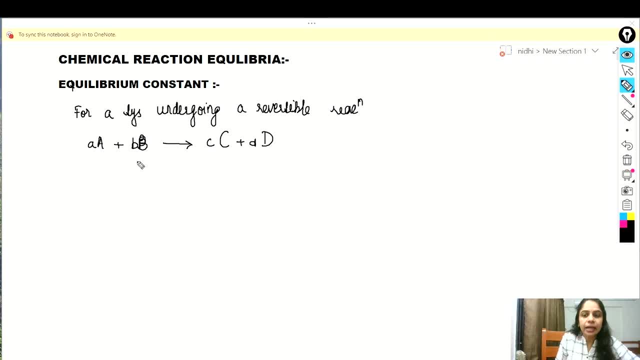 equilibrium constant is denoted by k and it is defined as the value of the reaction quotient. So when forward and reverse reaction occur at the same rate at chemical equilibrium, the chemical composition of the mixture does not change with time and the gives free energy. so change in Gibbs free energy is equal to. for the, that particular reaction will be equal to the zero. 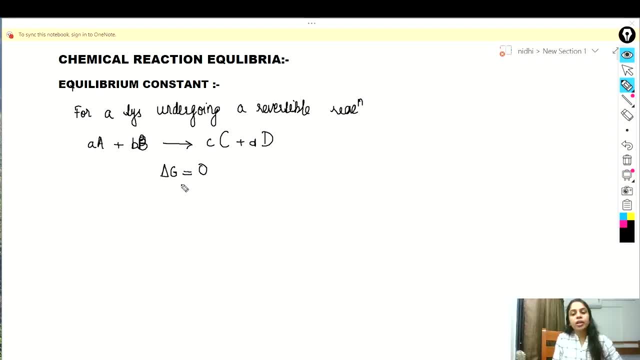 if the, if the composition of of a mixture at equilibrium is changed, then addition of some or, you know, if there is some addition of any reagent, a new equilibrium position will be reached. okay, so, every time, when, whenever we add some reactants, right, so we achieve, or we? 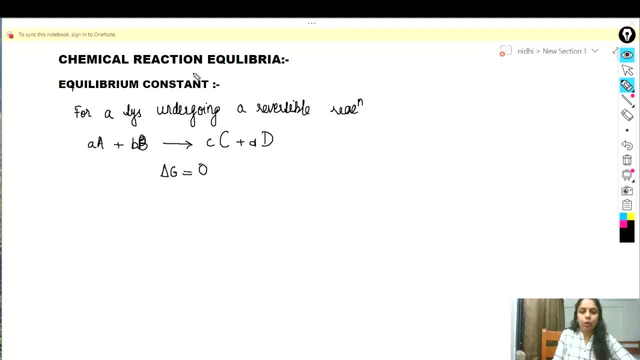 reach to a one new equilibrium state. okay. so k and k for this. let's take, this is the equation one. so for the really reaction, one is defined in terms of activity of reactants and product. so k, which is equilibrium constant, or ka for the activity. okay, so here what we have: ratio of product over. 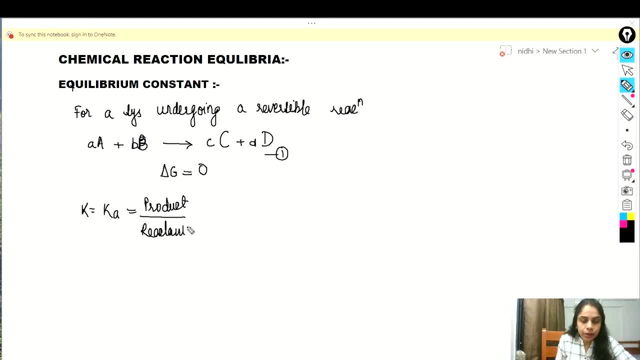 reactant, right, product over reactant. so how we can write this see. so here we have: uh, this is a, this is the activity. okay, in terms of activity, so products, so capital, c, and this is a stoichiometric coefficient. is that as a exponent, fine, then activity? 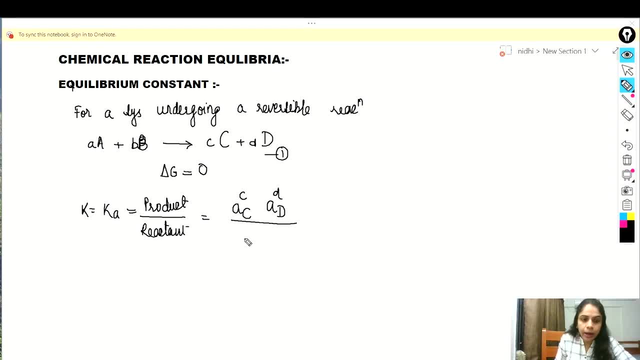 capital, d, small d, divided by activity of this and b, b, okay, and a is what? activity of pure component? ai, right, activity of pure component, which we know that activity of pure component, i fine. so how we can write this when it is in the ratio. so summation of a, i and stoichiometric coefficient. how we can define new. 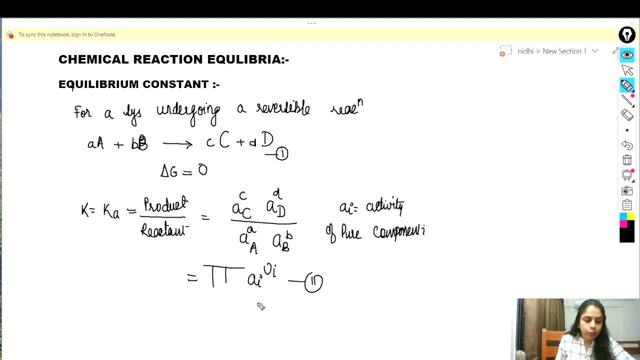 i, a i newer. let's take- this is equation number two. so we know that a i is the activity of component i and new i stoichiometric coefficient of this is what stoichiometric coefficient of stoichiometric coefficient of component i. so now we know that activity is the ratio of locality. 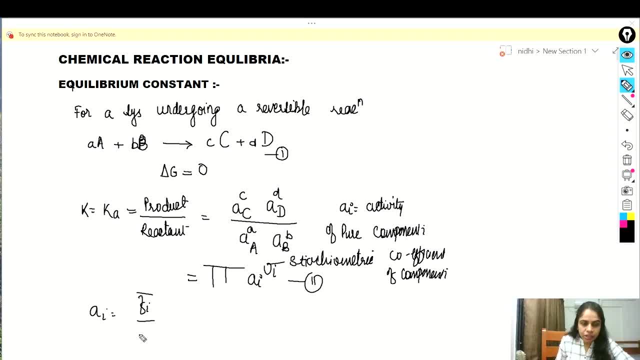 uh partial fugacity into the over uh partial fugacity of component i over fugacity at the standard stage. so this is the full elasticity of component. partial means we know that puedasity of component i in mixture and this is the fugacity of component i at a standard stage i what we see here is the actual diversity. 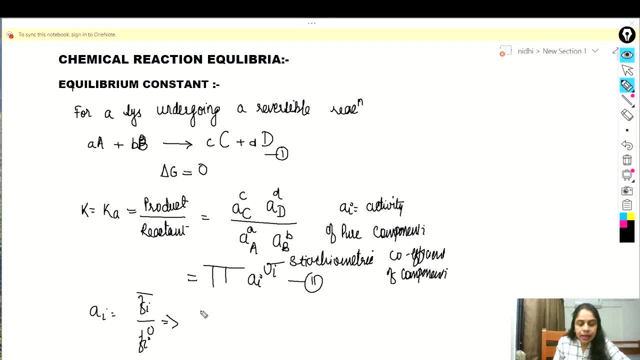 standard state. fine, So how we can write this: k is equals to k, a summation of f i over f i, not exponent of stoichiometric coefficient, and this is now defined by new term which is called k f right. So this is a equilibrium constant in terms of fugacity. We have k f summation of. 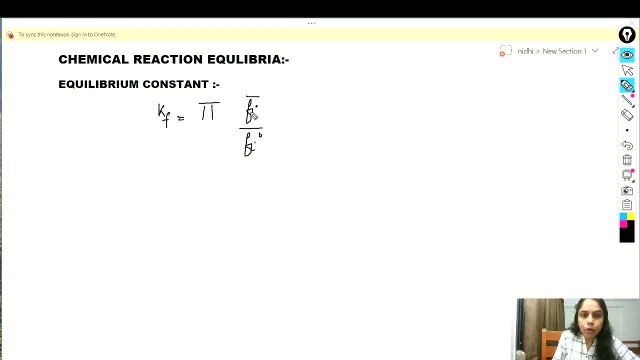 f i bar upon f i not nu i fine. At a standard state, fugacity of any pure component is equals to 1.. So f i not is equals to 1 fine. Therefore k f has become summation of f i bar nu i fine, Let's. 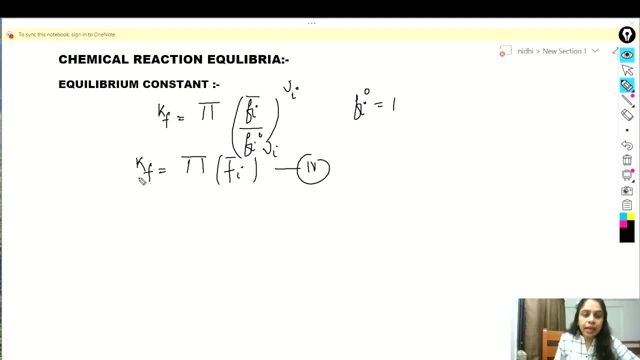 take this as the equation number 4, where k, f is equilibrium constant in terms of fugacity of component Fine, and for liquid and solid, the equilibrium constants are not numerically equal as a standard state because fugacity are not unit at that time. okay, Now another equilibrium constant. 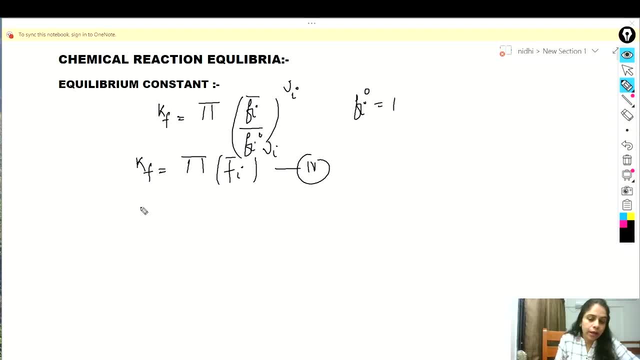 which is frequently used in the study of gaseous reaction, is k, p. So here we can just write down in terms of partial pressure. So p i bar nu i. Let's take this as the equation number 4.. Fine, okay. So now, using the relation fugacity coefficient, phi i bar is equals to f i bar upon. 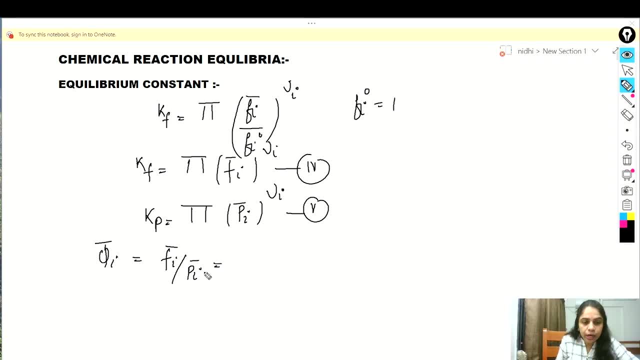 p i bar, which is the partial fugacity of component i, and this is the partial pressure of component i. So rearrange this. Therefore we get: f i bar is equals to phi i bar, p i bar. Let's take this as equation number 6.. Fine, So now from equation number 4 and 6.. 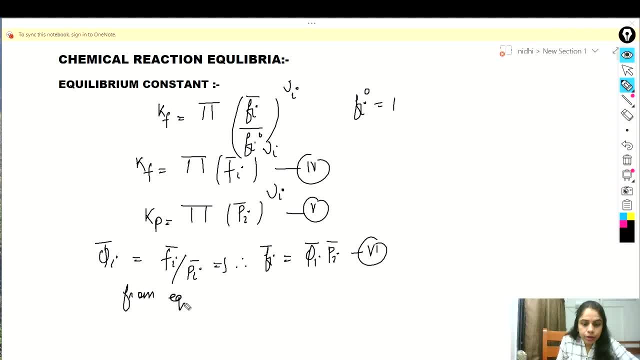 From equation 4 and 6.. K f is equals to, in place of f i, what we substitute: phi i bar p i bar nu i. Okay, And this will equal to phi i bar nu i p i bar nu i. So this is equal to phi i bar nu i, p i bar nu i. That's excuse me, This is not negative, So let's take this as the equation number 0.. Fine, So now using the relation fugacity coefficient: phi i bar nu i. Let's take this as the equation number 4.. Fine, So here we can just write down in terms of partial pressure: So k f is equal to f i bar nu i. p i bar nu i. That's excuse me, This is not negative, So let's take this as the equation number 4.. 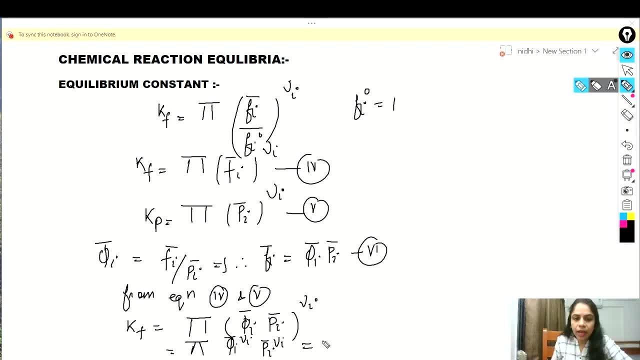 okay, this is what this is the fugacity equilibrium constant at. in terms of what? in terms of fugacity coefficient, and this is what k p in terms of pressure. okay, so k f is equals to k. f is equals to k phi k p. so this relation is applicable for gaseous system. if gas behaves ideally, then 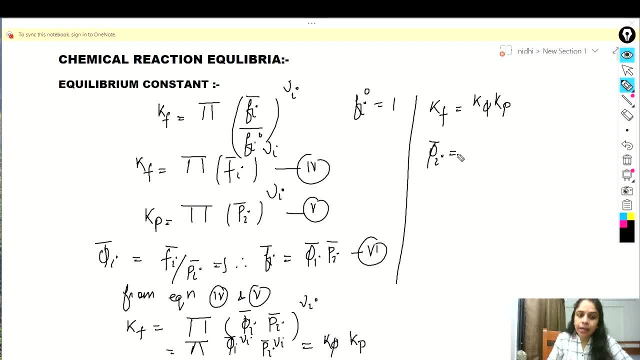 if gas behaves ideally, then phi i bar is equals to f, i bar upon p i bar is equals to one right. so then k is equals to k, f is equals to k, p, and this term will be equal to one. okay, so this is a one another relation. this is also one relation. so these are the some relations. 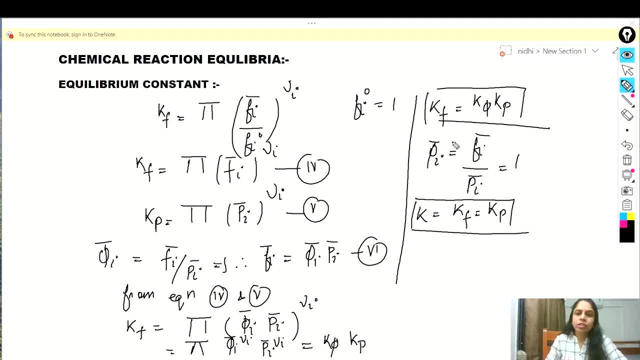 for equilibrium constant. equilibrium constant. there are different, many types of equilibrium constant and we can write equilibrium constant in different, different terms. just a bit: term up, use data given over. you can write in that term, okay. so the numerical value of equilibrium constant depend on. most important thing is in on form of stoichiometric equation, right in numerical value.